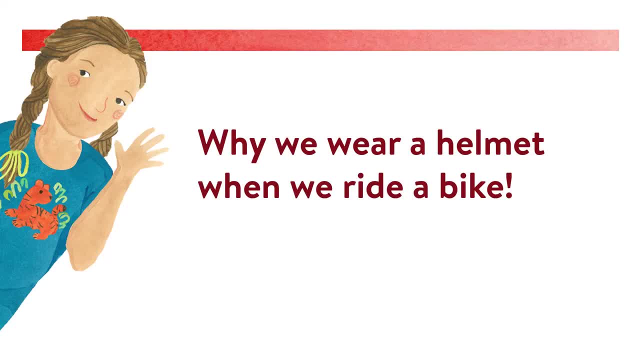 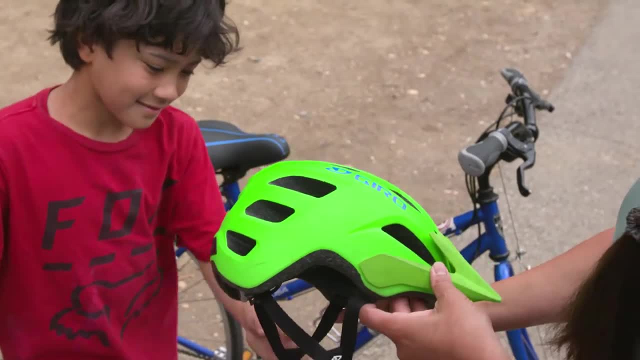 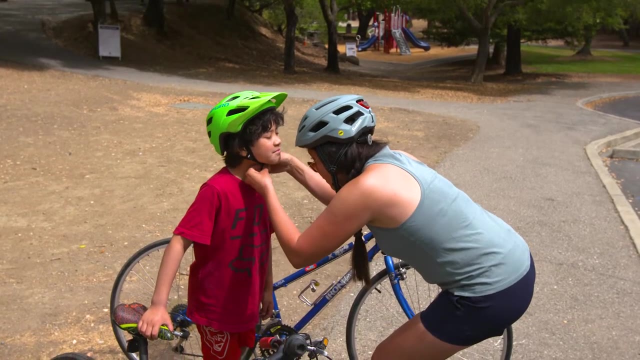 Your helmet is the first and best defense of protecting the brain. If your helmet has been cracked or damaged, it needs to be replaced. Now that you know how essential a helmet is to safety, let's talk about how to properly wear one. Your helmet should be the correct size for you. 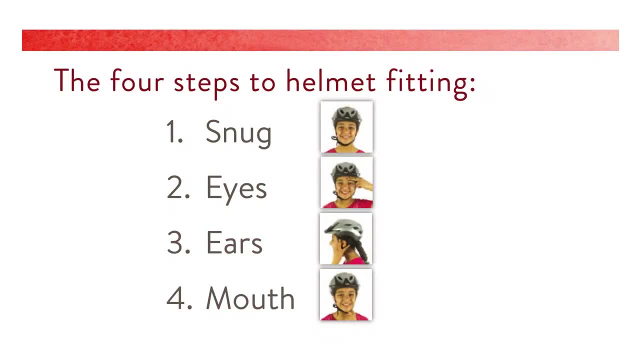 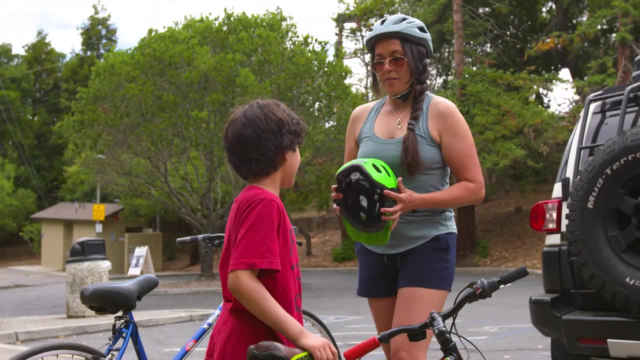 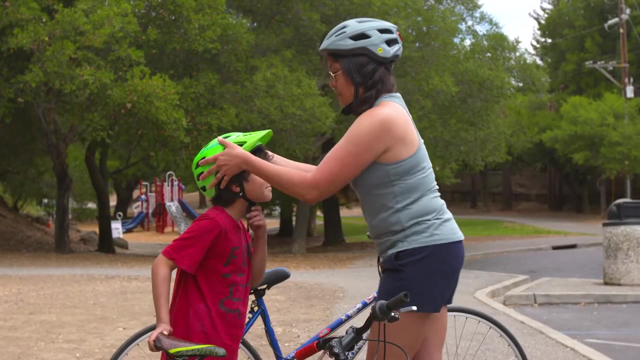 and properly adjusted. The four steps to check if your helmet is fitted correctly are: snug- eyes, ears and mouth Snug. Adjust the tension at the back of the helmet or replace the pad inserts if available, until the helmet fits snugly around your head. If you cannot get a snug fit, your helmet won't. 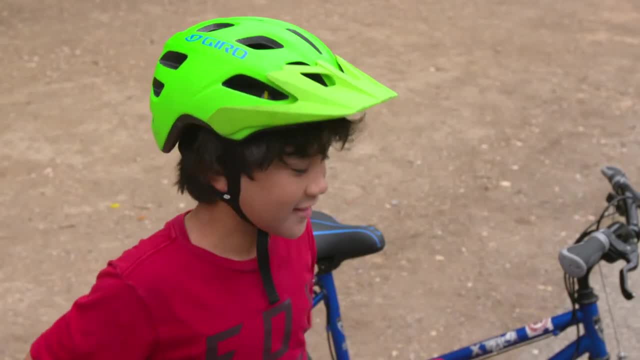 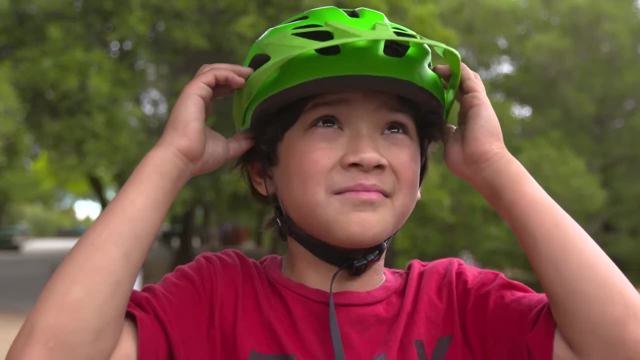 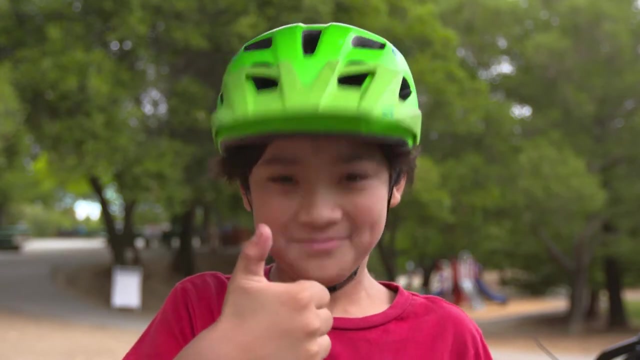 protect you in a crash, You may need to purchase a different sized helmet Eyes. Place your helmet level on your head so you're able to see the helmet rim when you look up. There should be no more than two finger widths between your eyebrows and the rim of the helmet Ears. 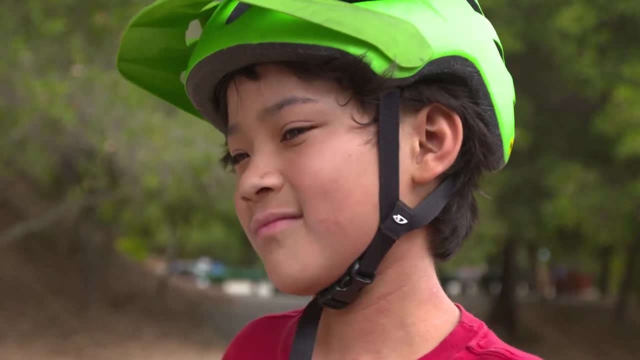 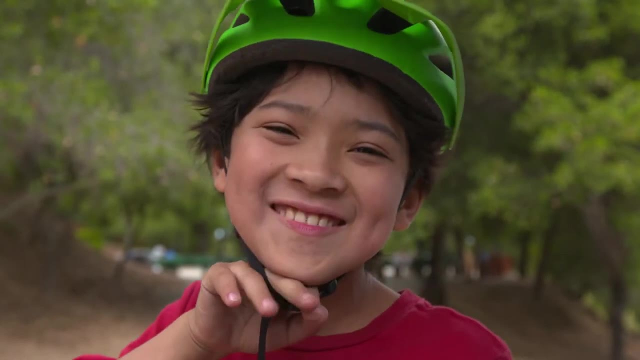 Adjust the straps so they make a Y that meets just below your ears Mouth. Adjust the chin strap so that no more than two fingers fit between the strap and your chin while fastened. Now that your helmet fits correctly, remember, wear the helmet for every ride. 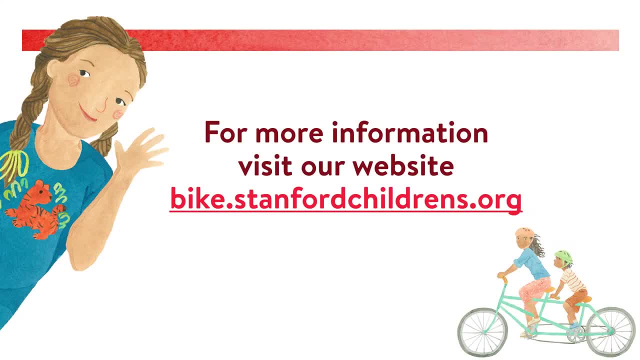 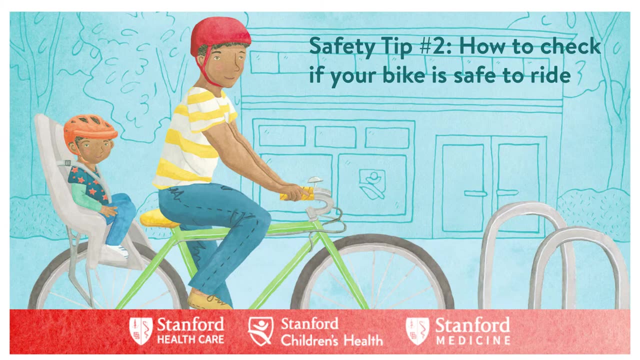 You can always refresh what you've learned today by visiting our website, bikestanfordchildrensorg. Safety. tip number two: How to check if your bike is safe to ride. After your helmet safety check is complete, we must make sure your bicycle is safe to start your bike riding. 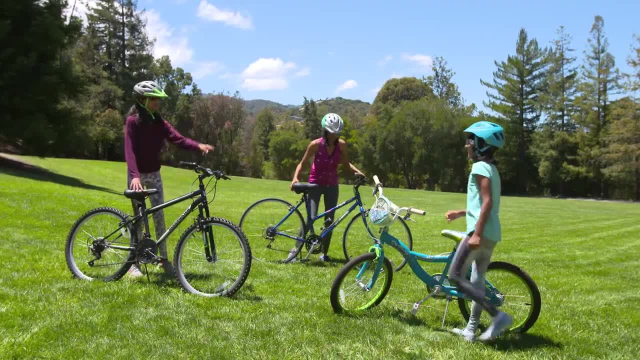 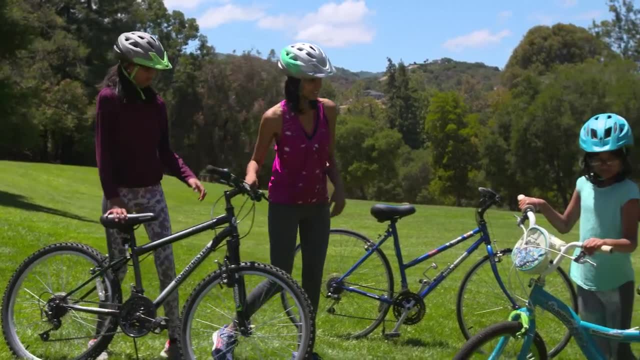 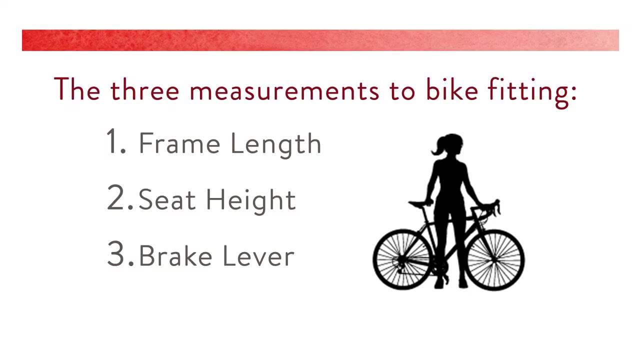 adventure. Your bike size matters and will affect how much control you have over the ride. A bike that is too big or too small can't be controlled properly and may be dangerous to ride. Make sure the bike you are riding fits you now. The following three measurements will allow you. 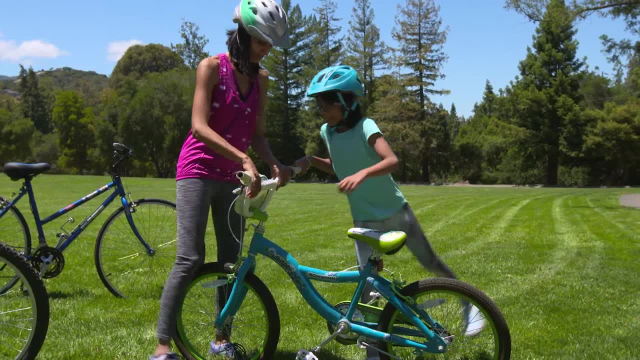 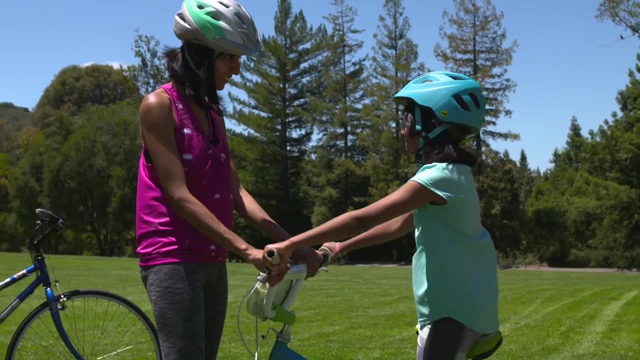 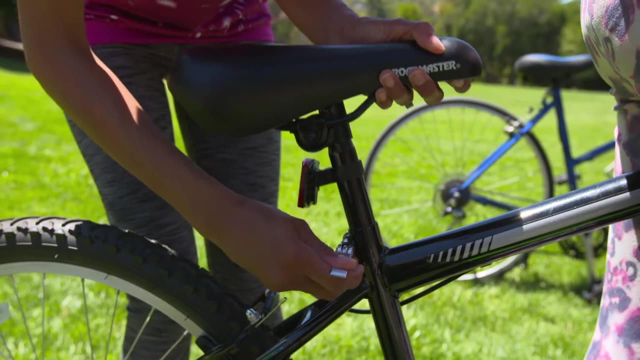 to see if your bike is the correct size. Measuring the frame length is our first step. You will need to position yourself on the bike seat and lean in to reach the handlebars. You want to avoid stretching out your back and shoulders. Next, we will need to adjust your seat height When standing in front of the seat with hands. 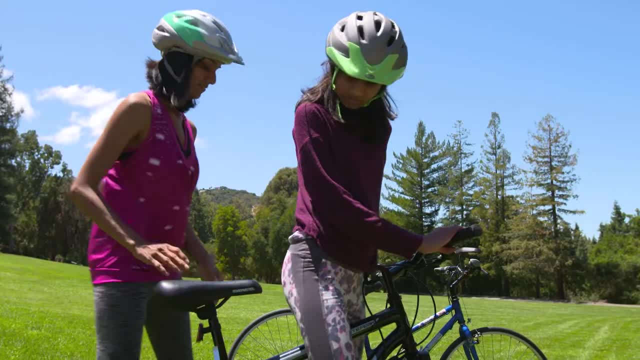 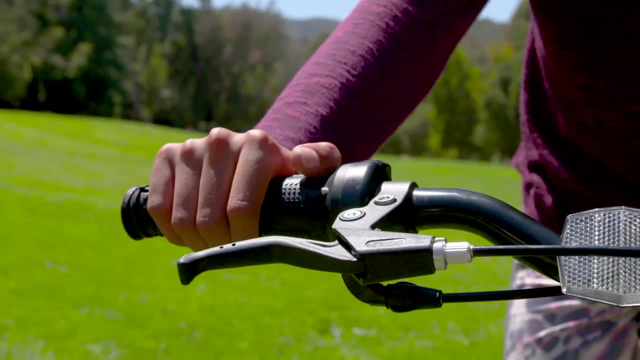 on the handlebar, you should be able to place the balls of both feet firmly on the ground. Lastly, we will check to see if you can effectively reach the brake levers From a seated position. reach to your brakes without stretching your back or shoulders and make sure you can pull them. 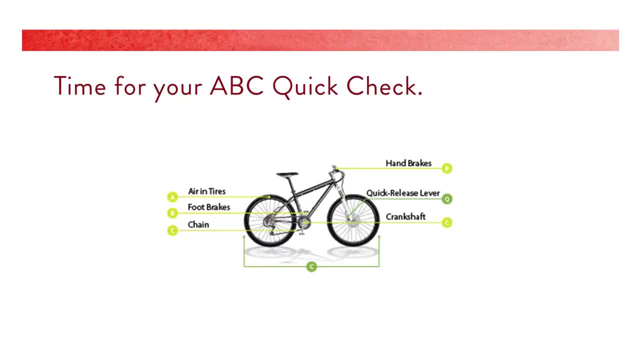 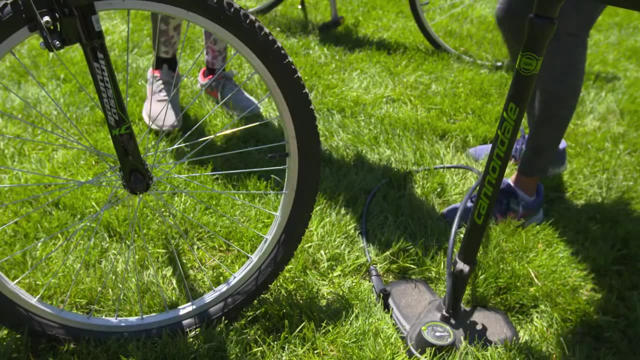 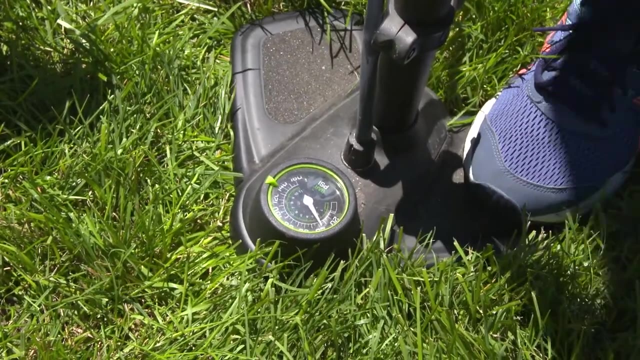 strongly. Now that your bike is properly fit, we can run through our bicycle ABC quick check. A is to check on the air pressure in your tires. You will need a pump to increase air pressure if needed. Some pumps come with a gauge to see how much air pressure is inside your tire. 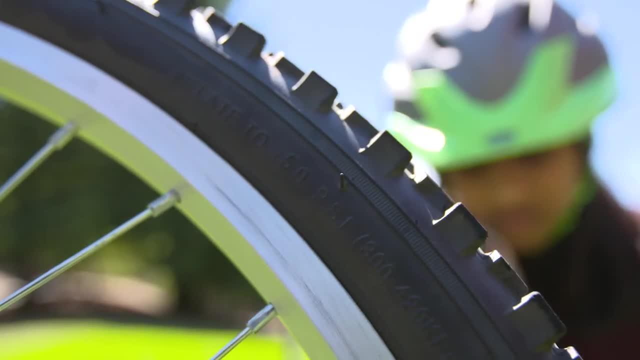 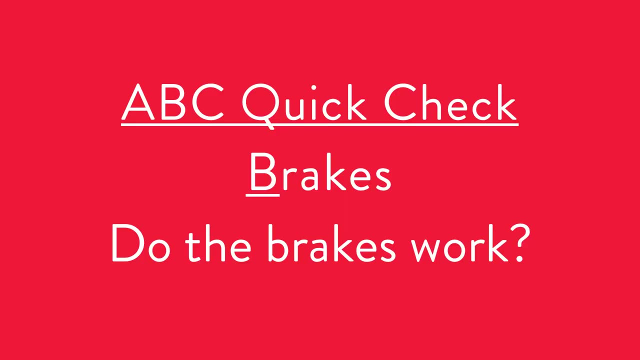 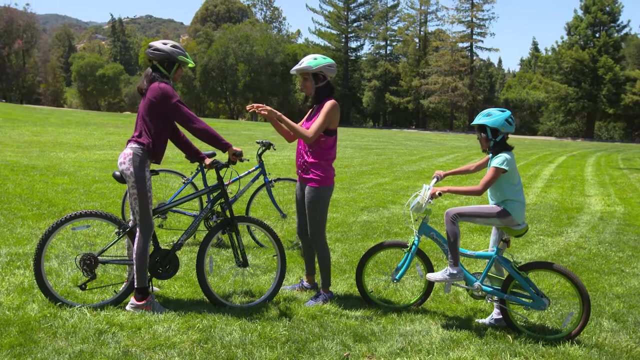 You will match this number with the recommended PSI number on the side of your tire. B is to make sure your brakes work. Even though this is second on our ABC quick check, it is the most important. Brakes that do not work effectively can put you in dangerous situations. 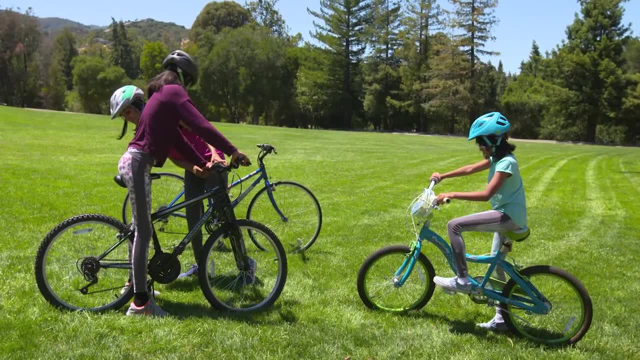 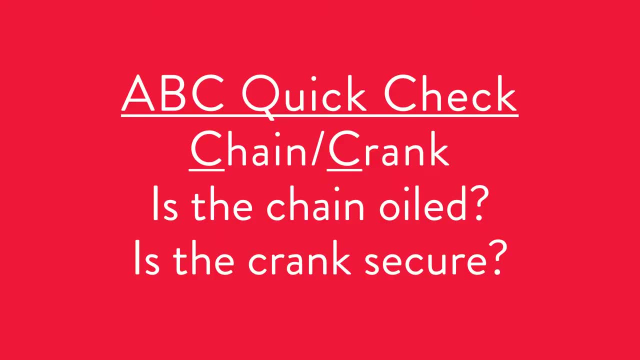 Squeeze on the brake levers, one at a time. Your left lever controls the front brake and your right lever controls the back brake. C has two parts: chain and crank. These parts are how you move your bike forward and must be taken care of to make sure your bike is in the right position. C has two parts: chain and crank. These parts are how you move your bike forward and must be taken care of to make sure your bike is in the right position. C has two parts: chain and crank. These parts are how you move your bike forward and must be taken care of to make sure your bike is in the right position. 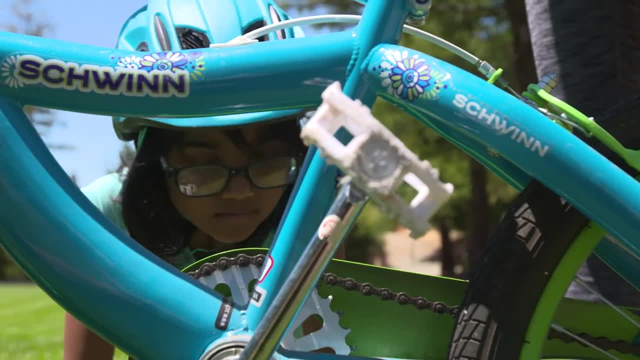 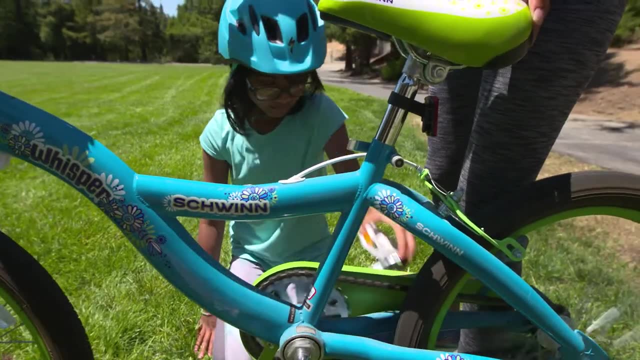 When checking your chain, look for any debris, dryness or rust. To check your crank, put one hand on your frame and one hand on your pedal. Spin your pedal forward slowly to check to see if the crank wobbles side to side. 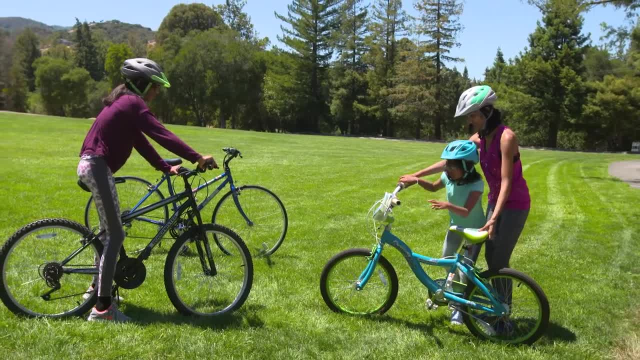 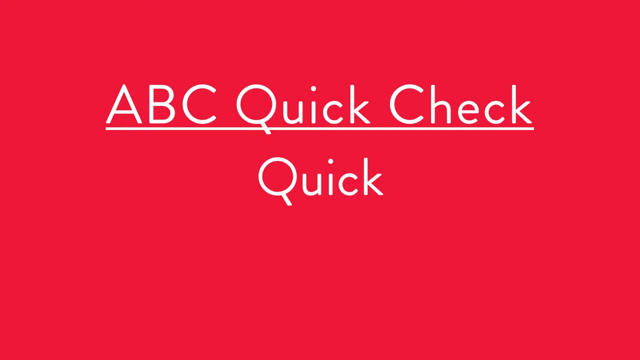 If you notice something wobble, ask your parent or an adult to tighten the crank. The ABCs are done. Time to move on to quick check. Quick. The quick release lever holds the wheels in place. Fastening this down will ensure that your wheels stay attached to the bike as you're riding. 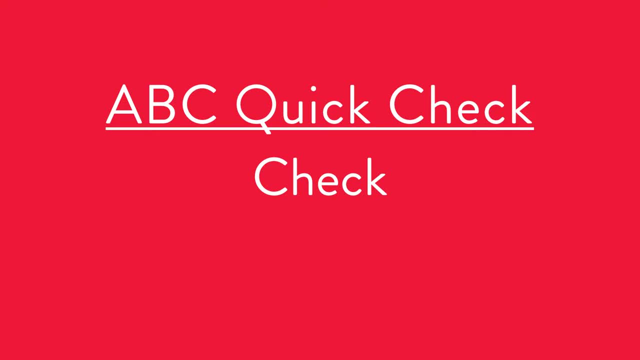 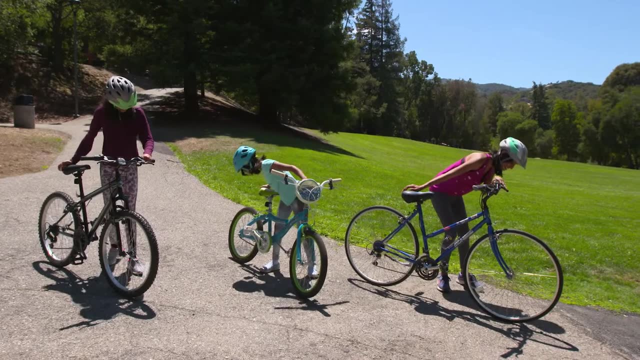 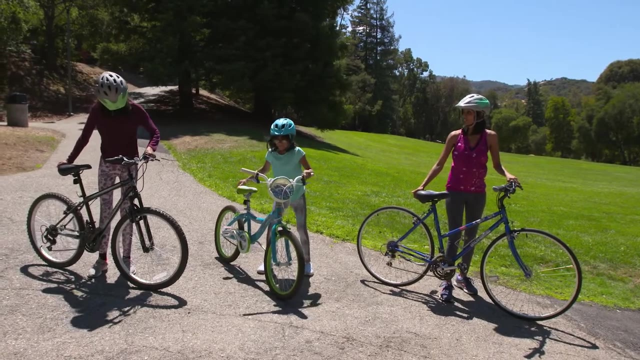 Check. This takes everything you just learned and puts it to the test. Now it's time to go on a slow ride to make sure everything is working properly. You will want to perform this test ride in an area that does not have traffic. Start your ride by putting on your helmet, Then make sure you're wearing bright colored or reflective clothing. 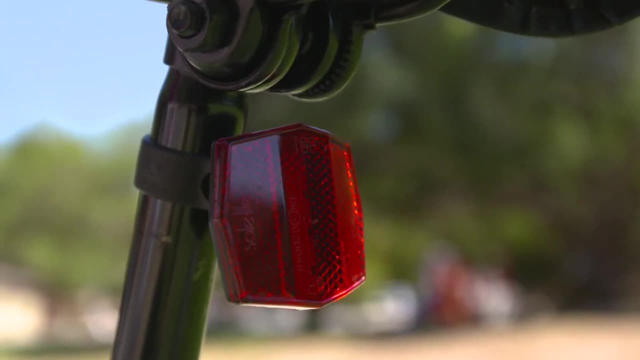 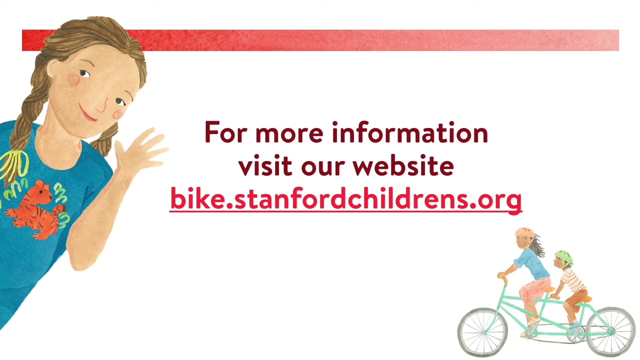 Equip your bike with a front white light or reflector and a back red reflector so that drivers can see you. You can always refresh what we have learned today by visiting our website, Bikestanfordchildrensorg. Safety tip number 3. Rules to follow while riding. 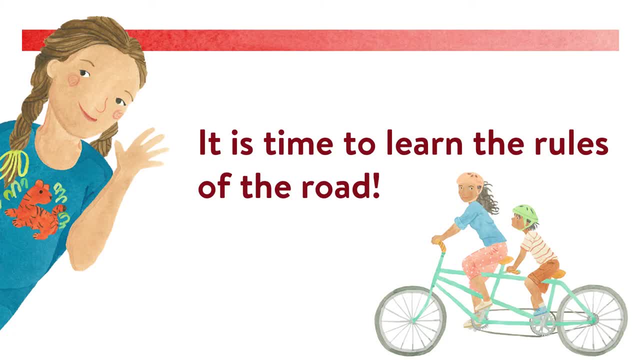 Now that your helmet and bicycle are safe and are working correctly, it's time to learn the rules of the road. Bicyclists follow the same rules as drivers. It's IMPORTANT, for example, because your bicycle is keeping thebart off the bike's rear. The bike is not turning鹜. 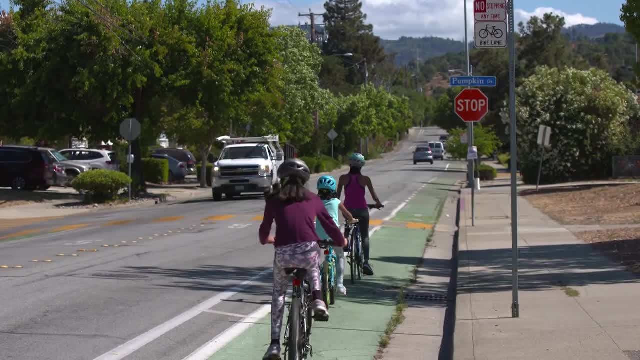 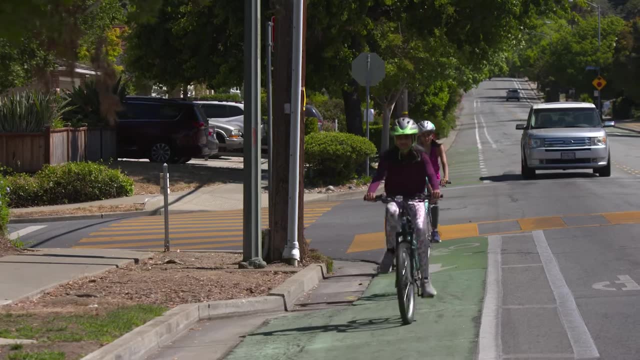 important to ride in the same direction as cars on the right side of the road following traffic. Riding in a bike-designated area is also important. Streets with a bike lane are marked with a solid white line. You want to ride inside that lane, as cars will be looking for you there. 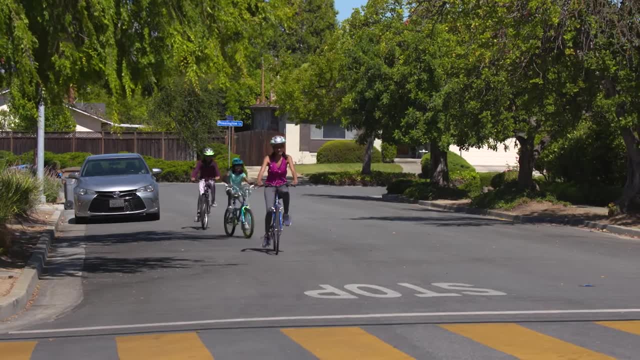 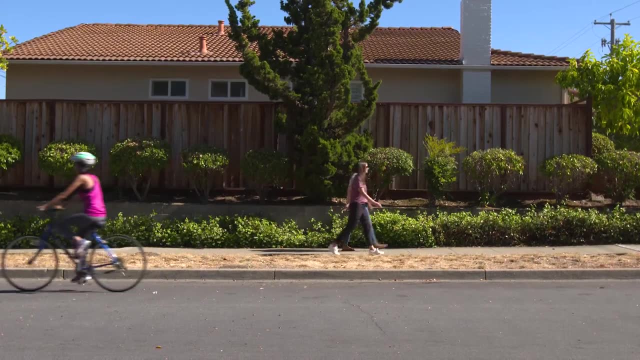 Focus on riding in a straight line in the bike lane. When riding on the street, you want to be seen and predictable. Do not ride on the sidewalks. That is where pedestrians are walking at a much slower speed than when you're riding. If you need to exit the bike lane or come 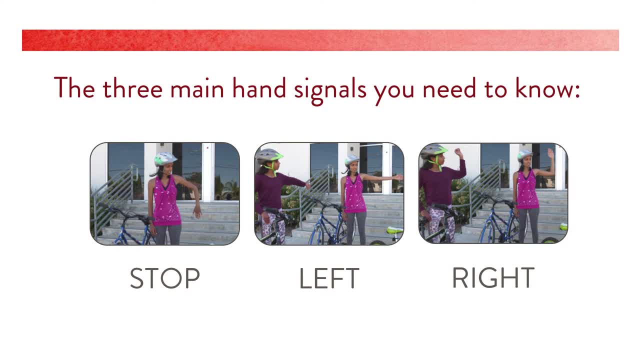 to a stop. there are three main hand signals that give the traffic around you a heads-up on what you're going to do. They are stopping, turning left or right. To signal stopping, extend your left arm out and bend your arm down at a 90-degree angle. 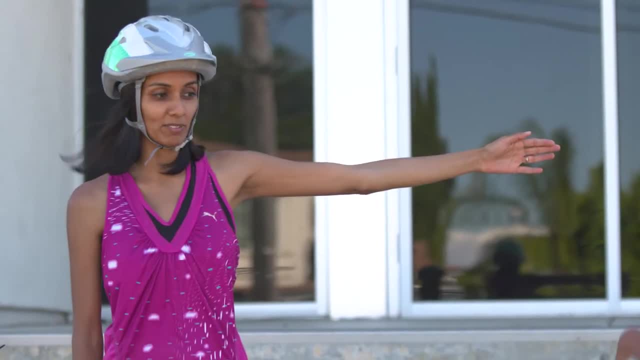 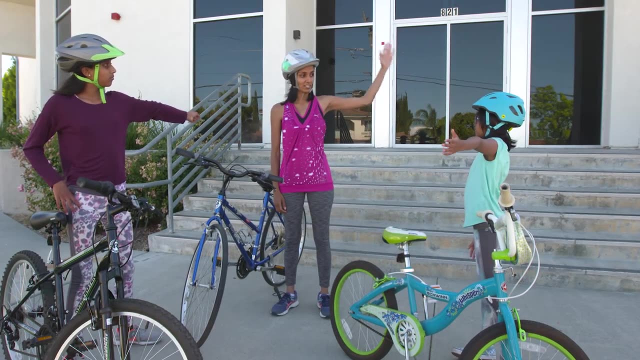 To signal that you're turning left, you will take your left hand and stick it straight out parallel to you To turn right, point your left arm straight out beside you and then bend your elbow to a right angle. Your hands should be pointing straight up towards the sky. 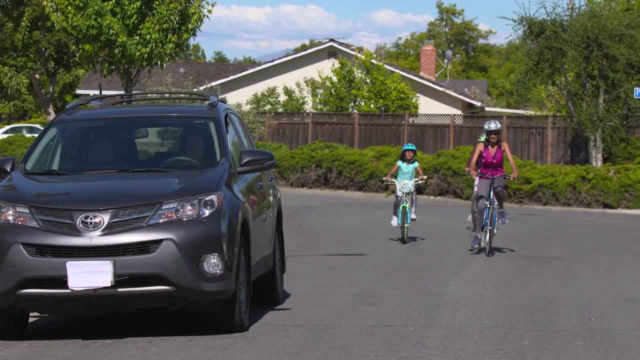 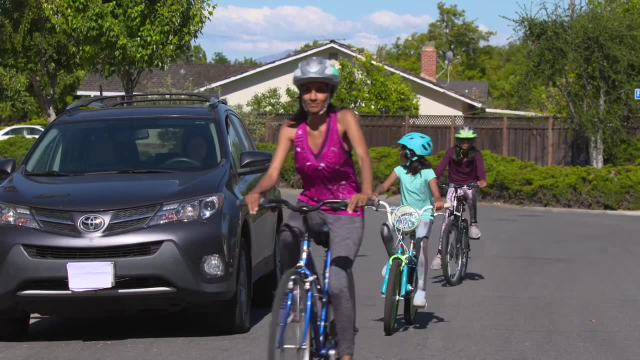 When cars are parked near a bike lane, you will want to anticipate their doors opening. This means it's a good idea to leave enough room to not be hit by a door if it opens. If you see a car parked on the side of the road with someone inside,